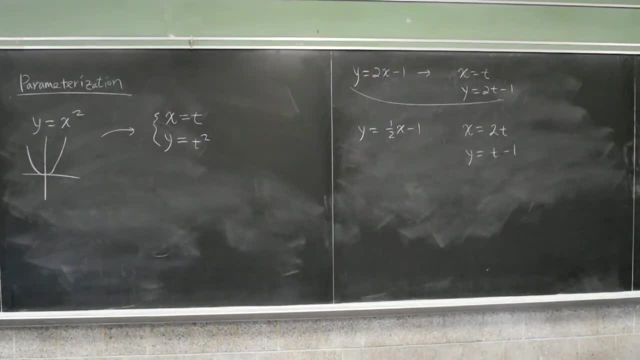 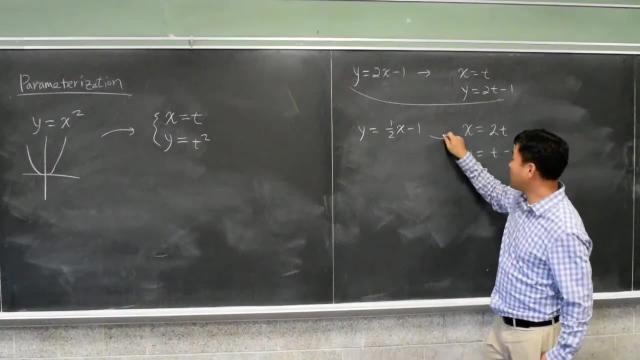 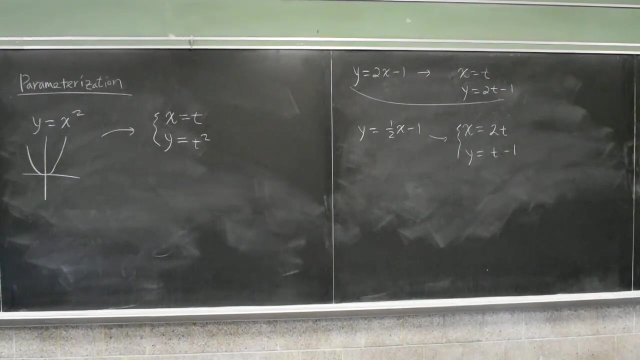 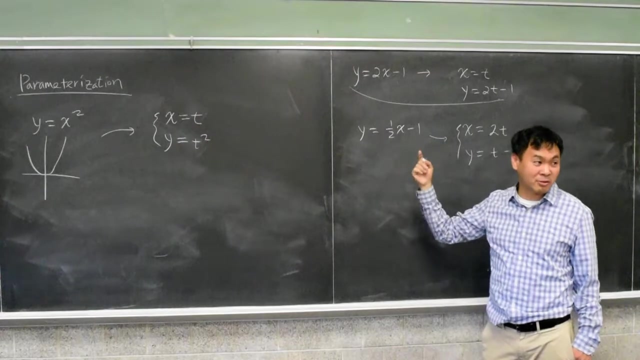 So that will be another parametrization, and before you had some fractions, now you don't, And sometimes that can help. It can help you in calculating other things And you may have noticed that, since you can take x equals to t, x equals to 2t or x equals to 4t, whatever. 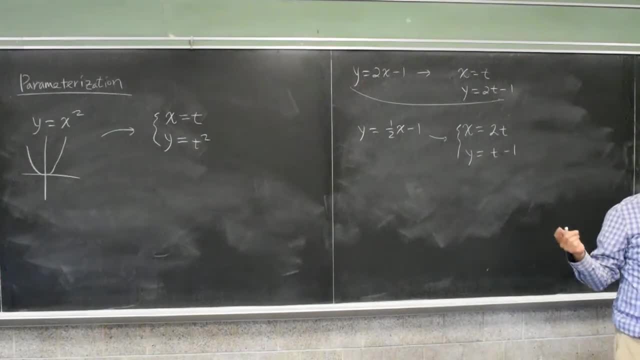 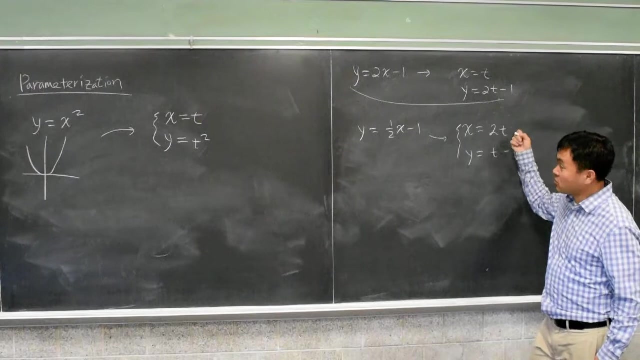 you can even take x equals to tangent of t if you want. So there are many different parametrizations you can come up with. So for any given equation between x and y, there are infinitely many different possible parametrizations that will give you the same equal graph. 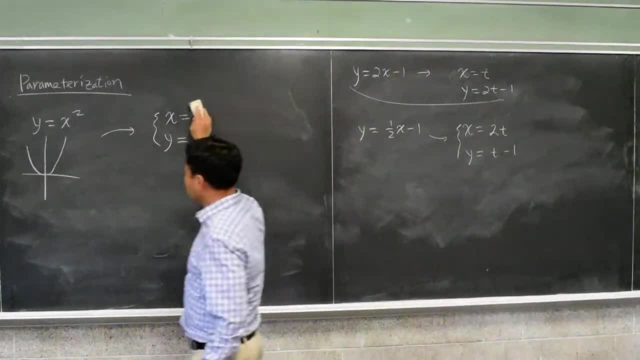 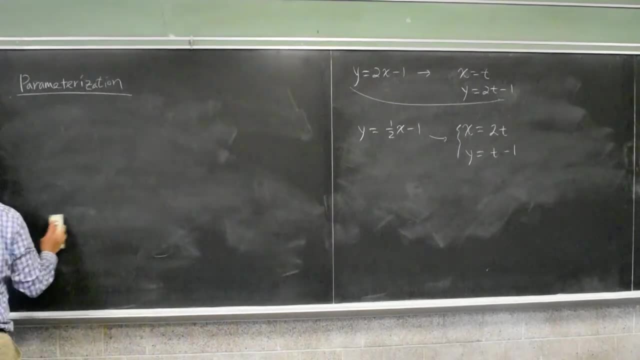 Now, however, there are some tricky ones that require some more attention, and these are the ones related to circles. So let's see, Let's start with the simplest one: the unit circle. The unit circle has the equation x squared plus y squared, equal to 1, and the problem? 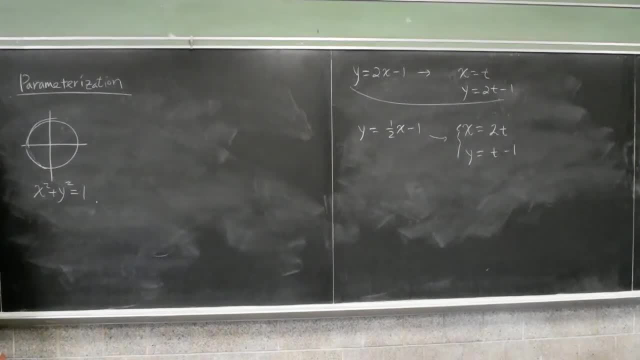 with just taking x equals to t is that y is not really a function of x, right? We learned that it fails the vertical line test, so it's not a function. So if you really try to set x equal to t, then you plug it in here and you get t squared. 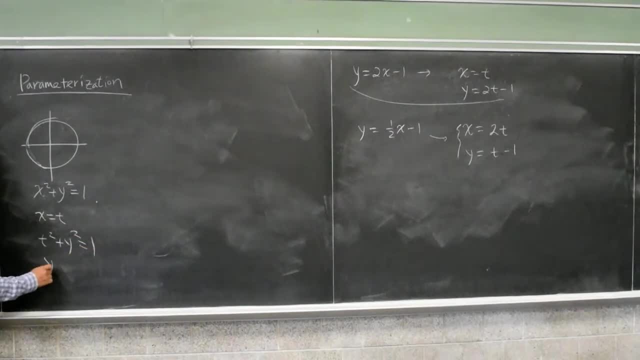 plus y squared equal to 1.. You subtract and you solve for y. you get plus minus square root of 1 minus t squared. And because you have plus or minus, the plus one will be parametrizing the top half circle. 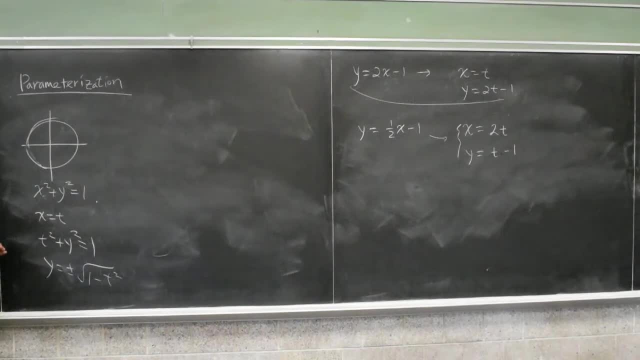 and the minus will only parametrize the bottom half circle, And this is not good, because you fail to parametrize the entire circle by a single equation. You need two equations, one plus another negative, so that's bad. So you need something very different and you start with something that's well-known. 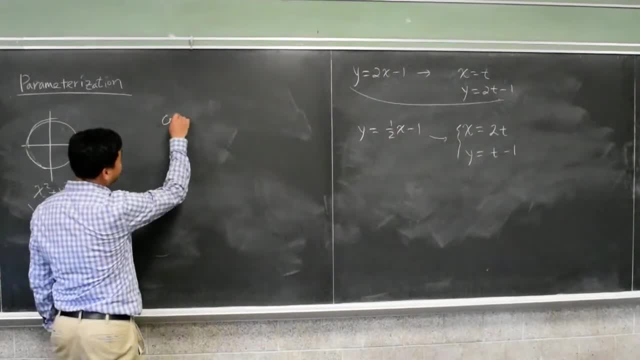 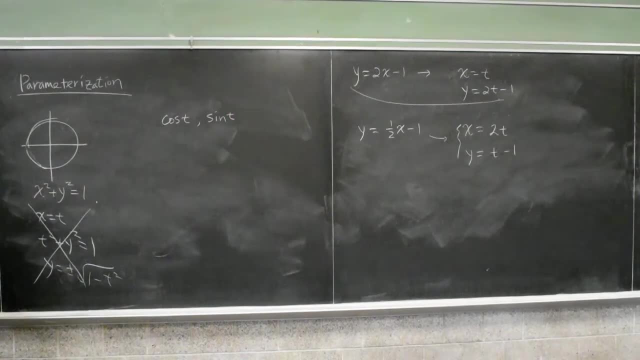 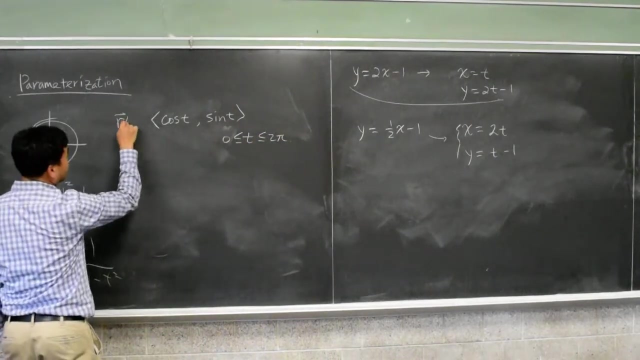 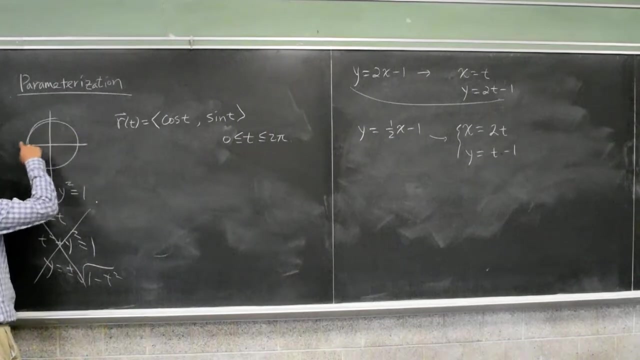 We all know that if you have cosine t, comma sine t, then these are the points on the unit circle right And t going from 0 to 2.. 2 pi that represents this circle where this particle is just going round and round right. 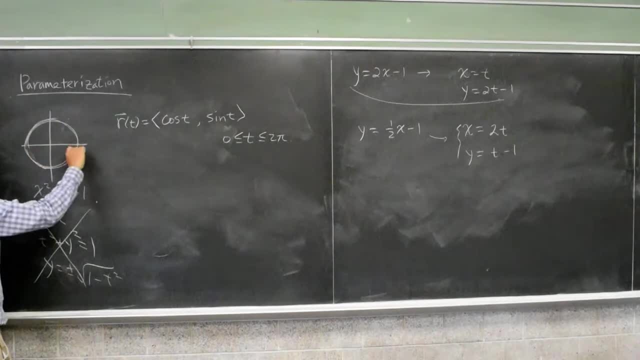 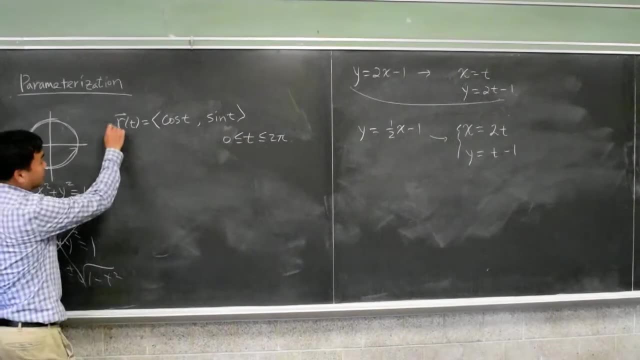 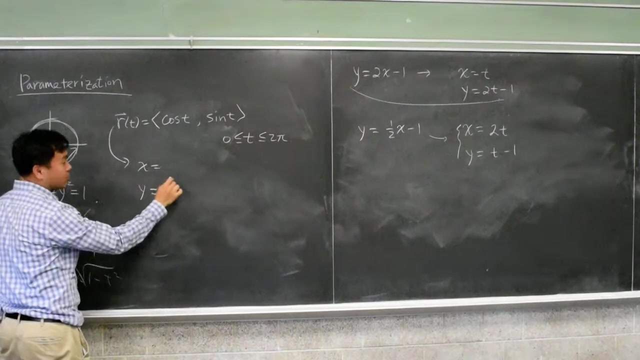 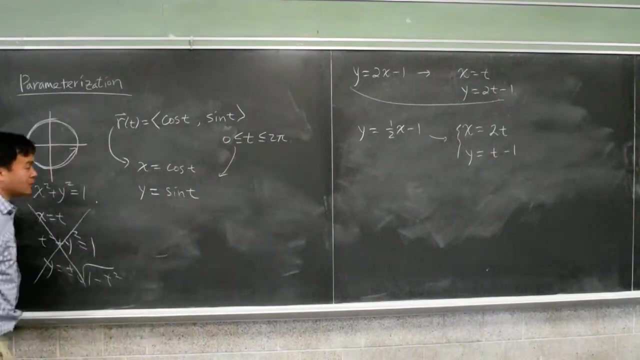 And this t is from 0 to 2 pi. it just goes round the circle just once, right? So we start from this Now. how would you write this in terms of x equal to something and y equals t, x equal to cosine t, y equals to sine t. with the same balance, right? 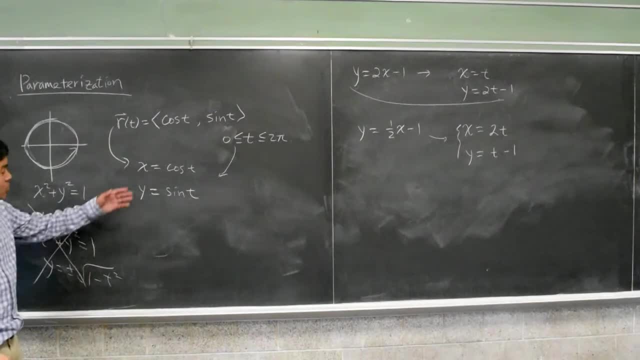 So that would be the parametrization. By the way, we call this the parametrization, but sometimes we also call this the parametrization, So you should be able to write both. And also, if you just see this, you should also think this. 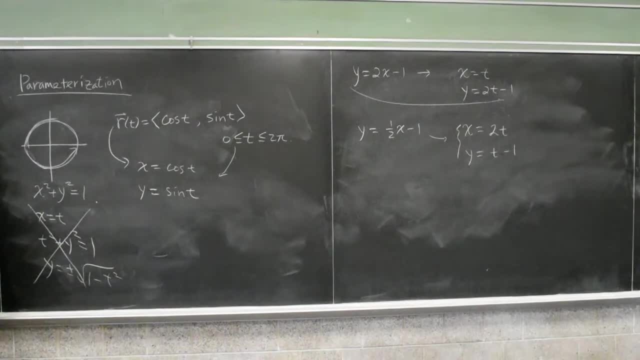 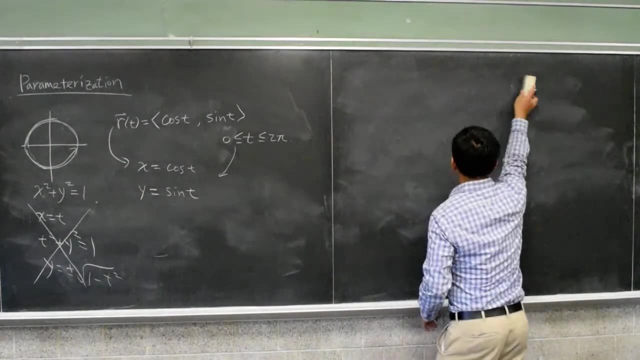 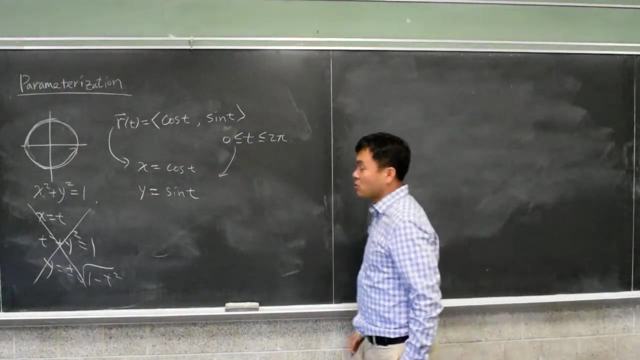 If you just see this, you should also think this: okay, Same thing Now. from there we can do some more variations Later on in this class. we're going to use parametrization to do integrations over some curves. 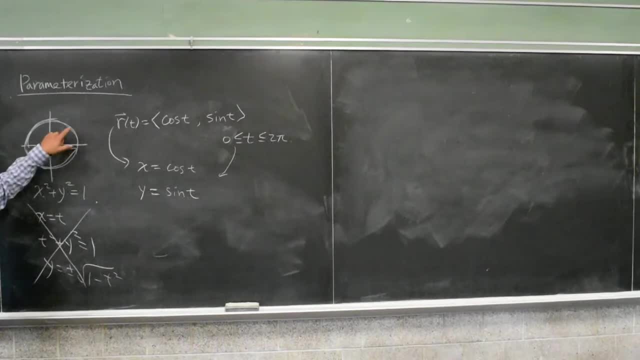 So if we have some quantity over this curve, we can integrate that quantity over the curve, And when we do this, we will have to parametrize. That's actually the real reason. we want to know how to parametrize Now in that section. 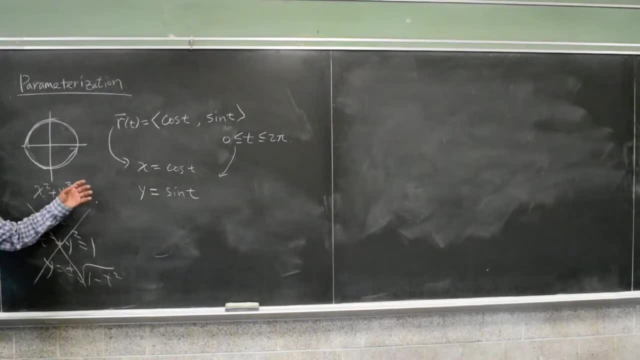 which we will learn later, which is called the path integrals, line integrals for that chapter. there's another important concept. The concept is orientation. Sometimes you want to parametrize this curve in the counterclockwise direction, or sometimes you want to parametrize in the direction that's clockwise. 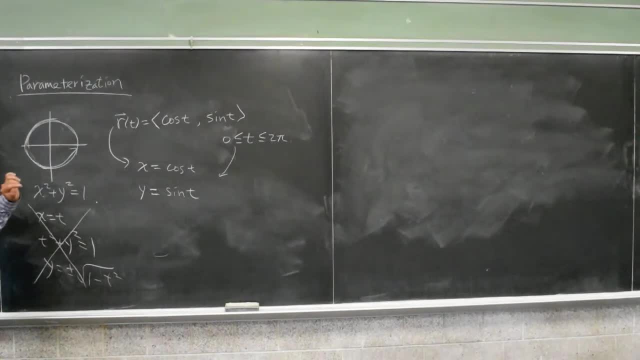 And you have to know how to parametrize in both directions. okay, So for this one, how would you make it go clockwise? So this is counterclockwise, right? How would you make it go clockwise? Any ideas? Yes, 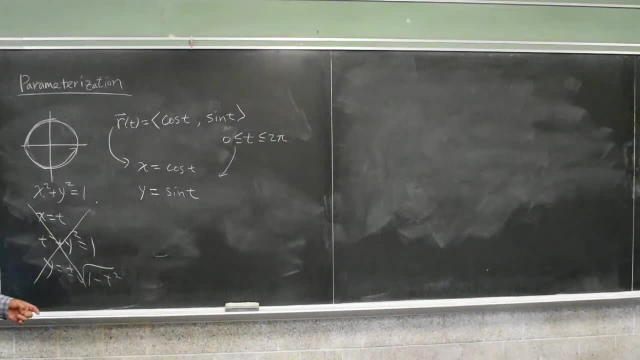 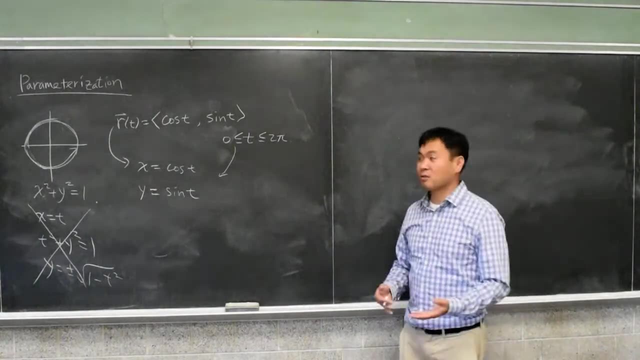 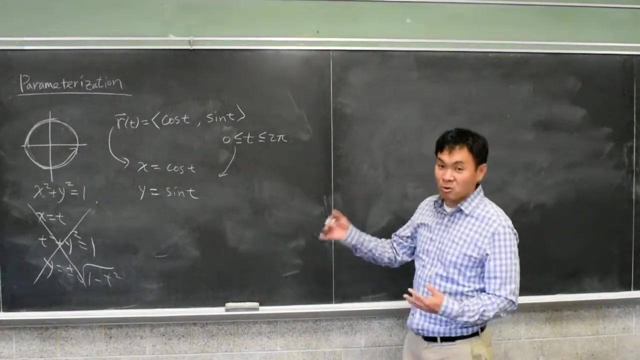 Switch x and y. Right right, So switching x and y. there are actually many different ways to do it. It's just like there are infinitely many parametrizations for the same curve. There are infinitely many different parametrizations that will make the circle go the opposite way. 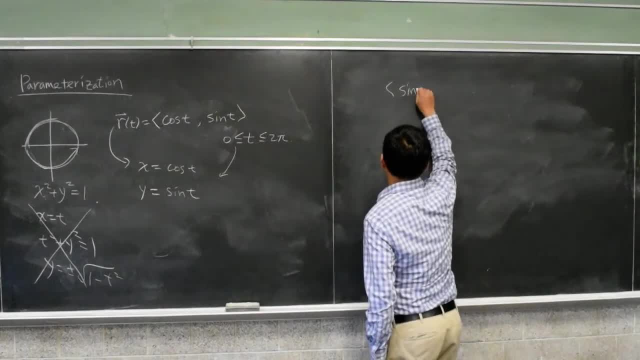 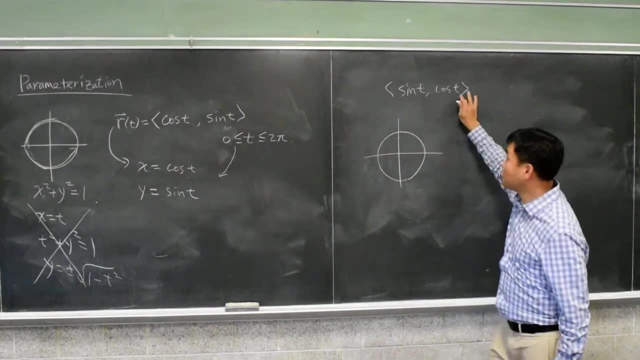 But one way to do it will be to switch x and y. You get sine t, cosine t. Now let's see why this is. If you plug in t equal to 0,, this is 0 comma 1.. So you're here. 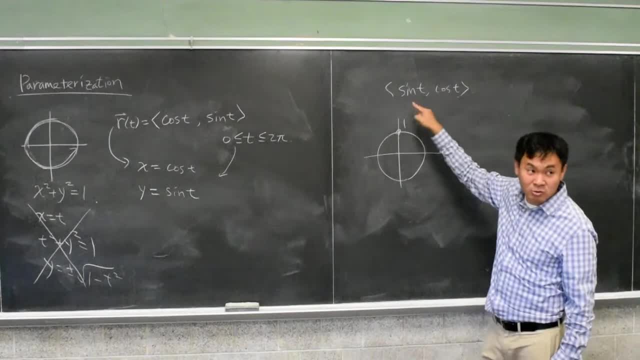 Now, if you plug in t equal to 90 degrees or pi over 2, when t is pi over 2, it's 1 comma 0.. Cosine of 90 degrees is 1, cosine of 90 is 0.. 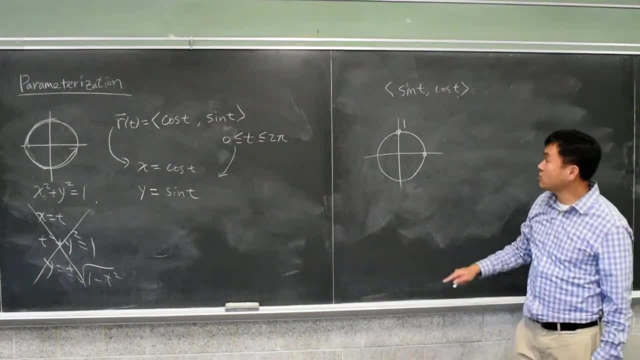 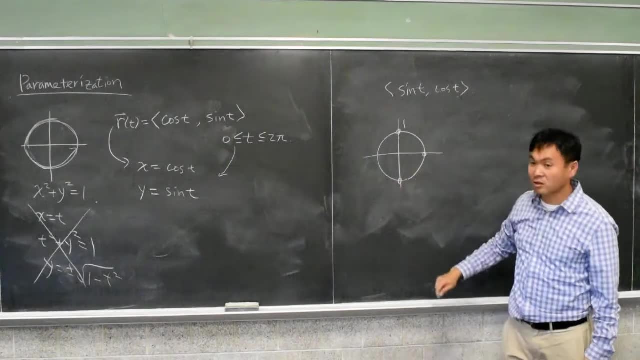 And then when t is 180 degrees, then sine 180 is 0, cosine 180 is negative 1, so you get 0 comma negative 1, which is here. Okay, So when t is 0, you're here. 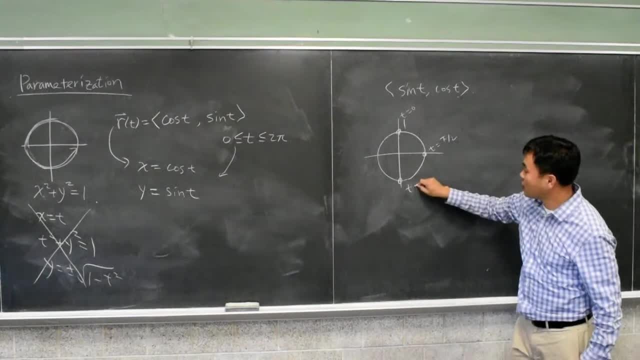 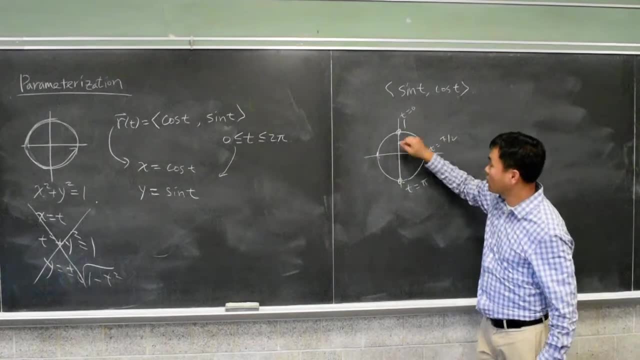 When t is pi over 2, you're here. When t is pi, you're here, And then you can try this for more numbers and you'll see that as t increases, it's going to go this way, going this way. 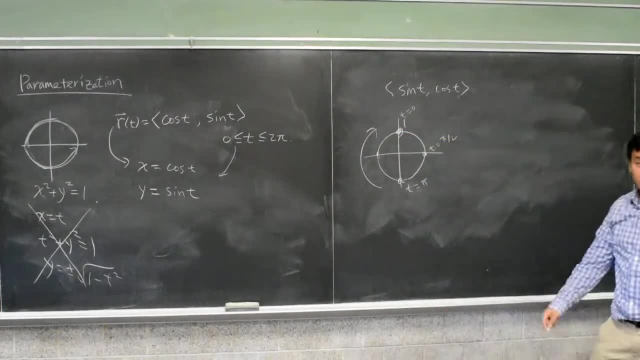 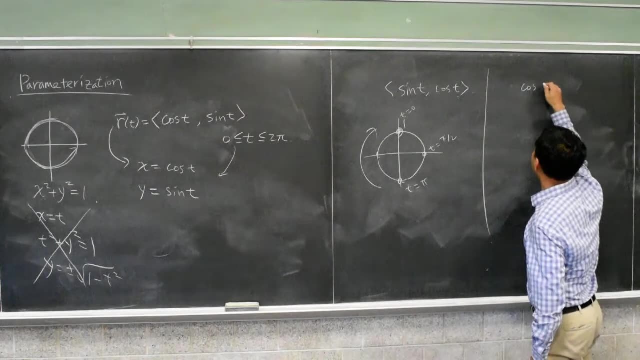 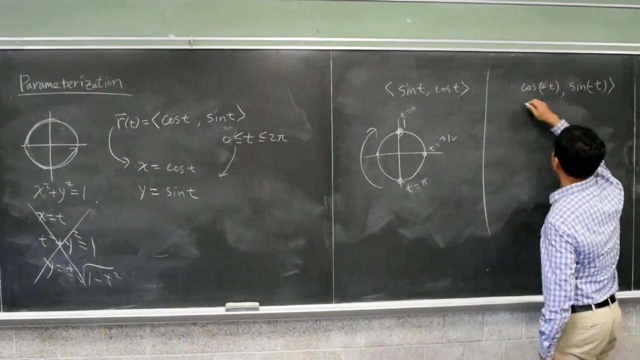 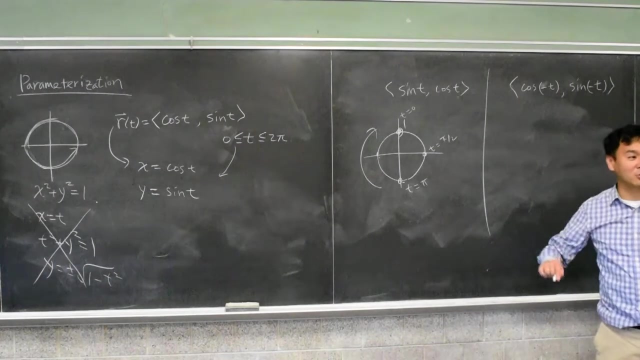 Okay, Starting Now, here's another parametrization that does the same thing. How about cosine of negative t, sine of negative t? So what you're doing is you're switching the sine of t. In that case, it also goes counterclockwise. 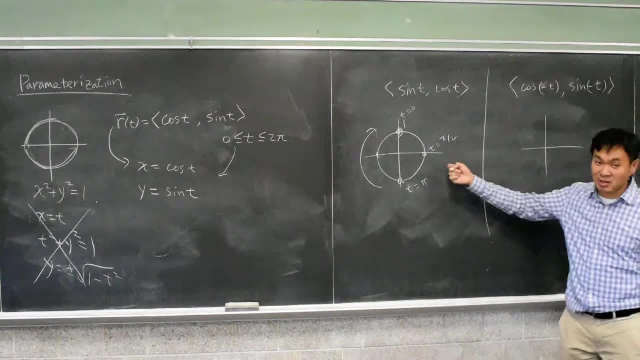 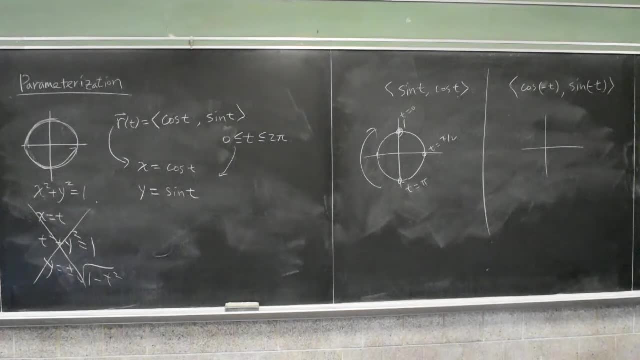 What's the big difference between this parametrization and that parametrization? in terms of the movement, They actually go around the circle at the same speed. What else can you see? Yeah, It starts at like 180 degrees, Right, So the starting point is different. 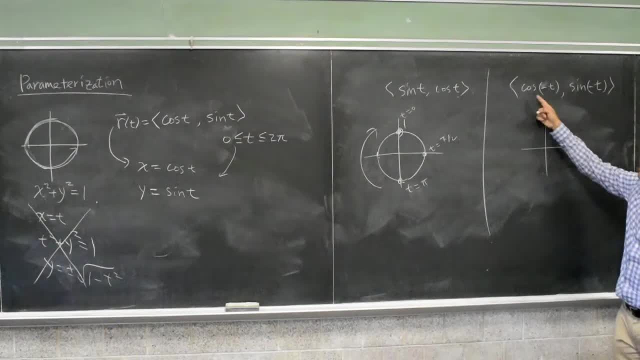 So the starting point is: if you plug in 0, you get cosine of 0, which is 1,, sine of 0, which is 0, so you get 1 comma 0. And when you plug in 90 degrees, this is actually cosine, is the even function. 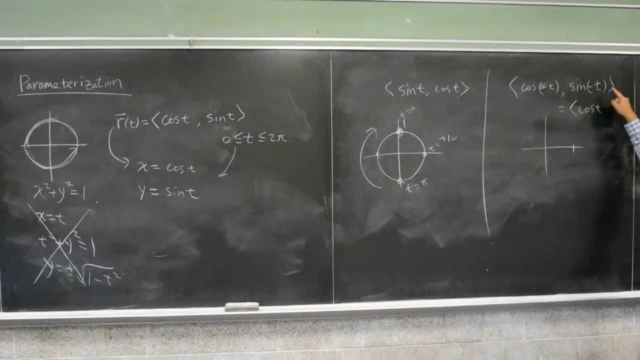 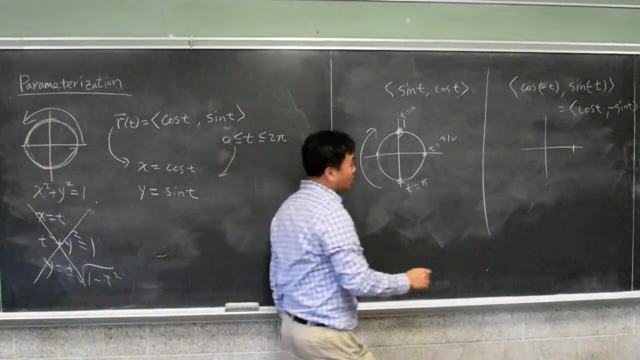 so that's the same as cosine t, whereas sine is an odd function. so sine of negative t, negative comes out right. So it's like a mirror image of this thing. So instead of going that way, it's going to go this way. 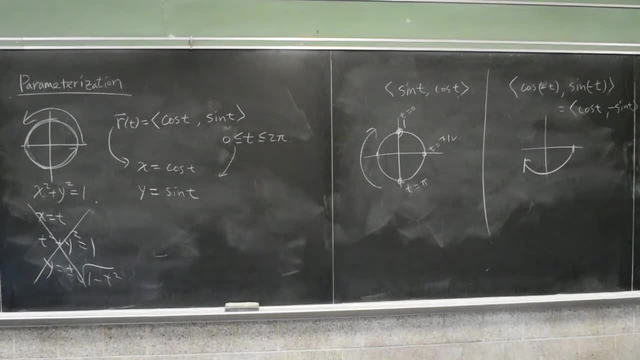 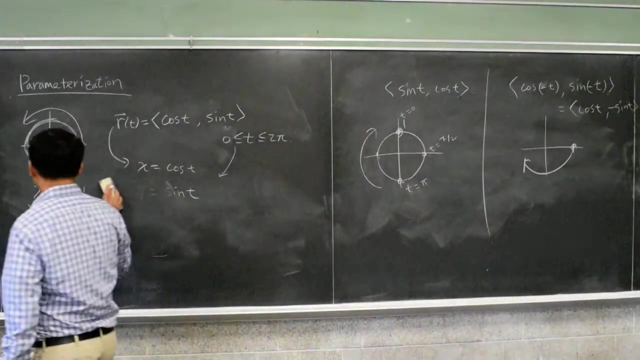 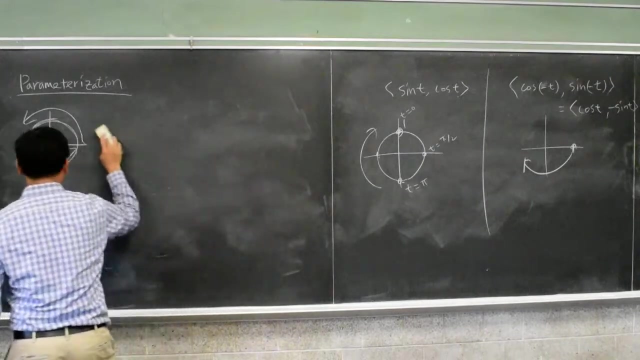 OK, Starting from here. So this goes clockwise, That also goes clockwise. The difference is: this one starts at 1 comma 0. This one starts at 0 comma 1.. Now, from here we can talk about many different kinds of circles. 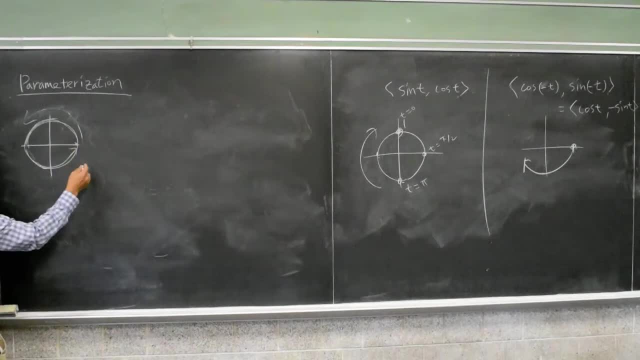 What if we have a radius 4 circle and we want it to go clockwise? What would be the parameterization? 4 cosine t. 4 cosine t 4 sine t. 4 sine t, 4 sine t. This is going to parameterize the curve so that it goes that way. 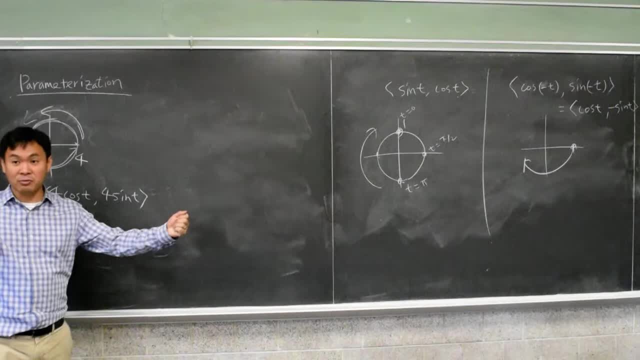 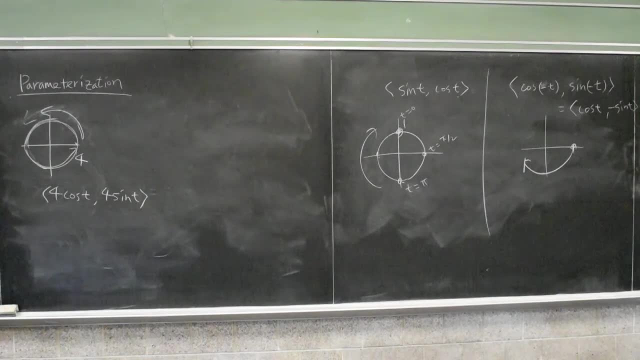 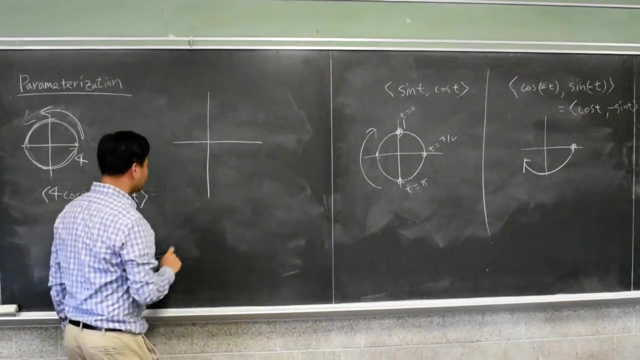 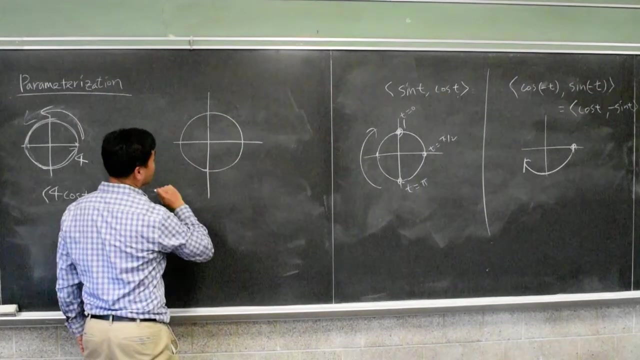 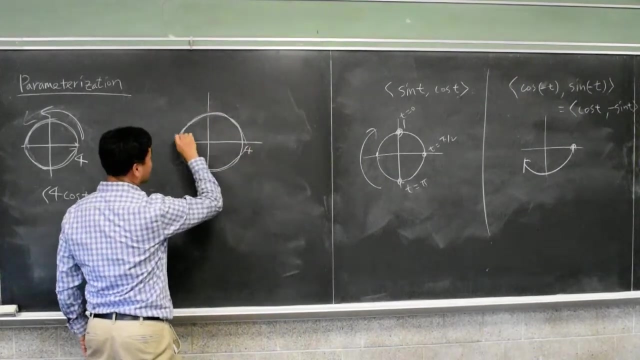 Because we multiply by 4, the entire curve will be multiplied by 4, so it will go around this circle of radius 4.. OK, Let's see another one. Sometimes you might want to do something. The circle is slightly squashed. 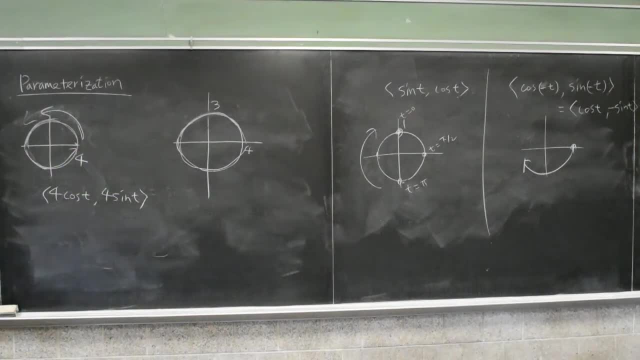 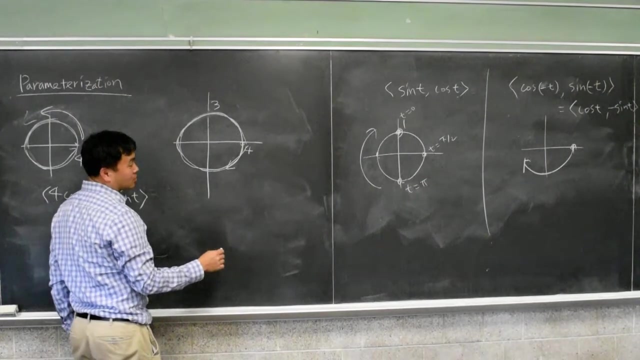 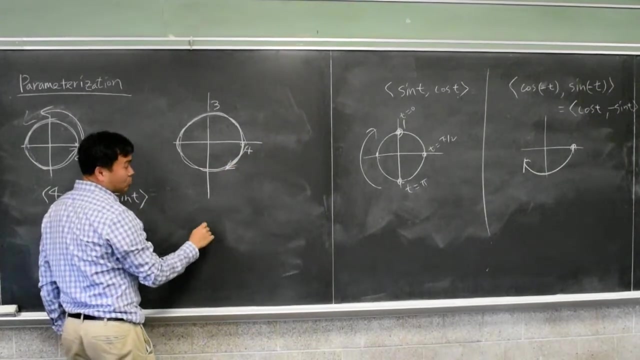 So let's think about this oval-shaped thing And let's say I want to move this way clockwise. What's the parameterization? I should use 4 sine t, 4 sine t. OK, So first, because I want clockwise, I should be using either one of those. 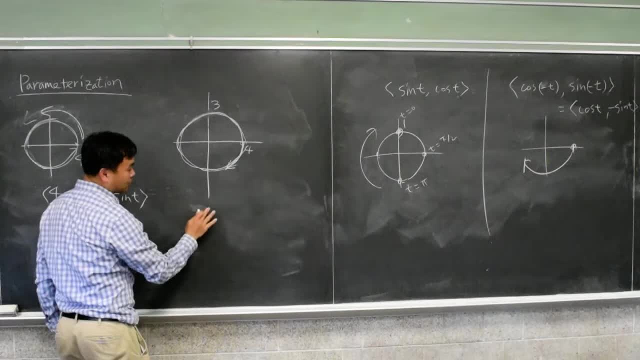 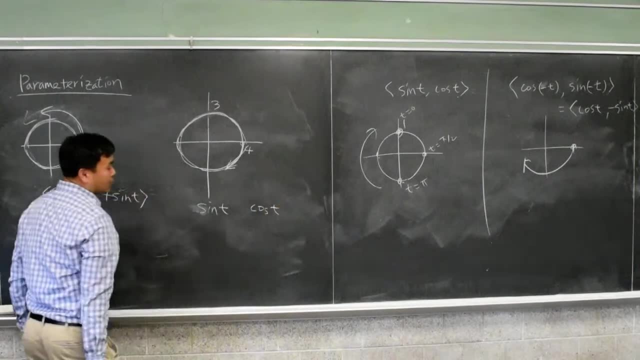 And you guys chose sine and cosine. That's good. So let's just say we used that one, sine t and cosine t, And then I need the x-coordinate to vary from negative 4 to 4.. So this should have 4.. 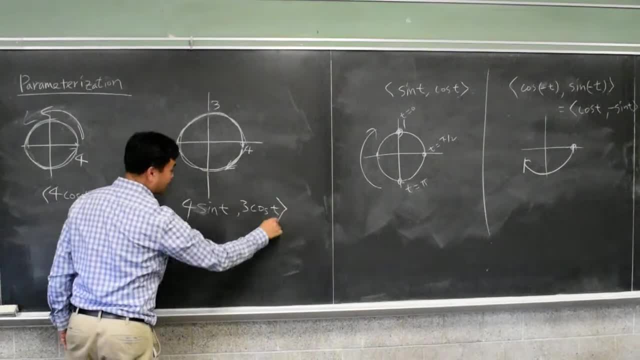 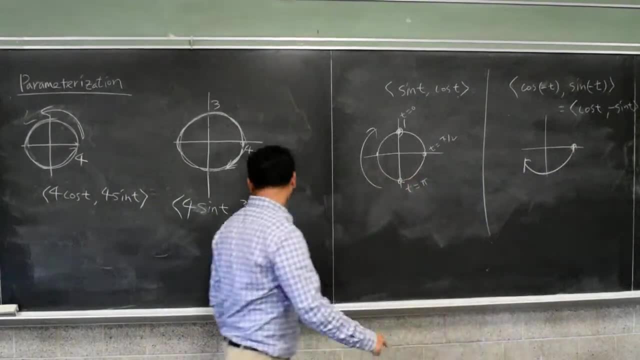 And y-coordinate should vary from negative 3 to 3.. So this should be it. So that's one possibility, Another one. if I were to choose this one, then I would be using cosine t, sine t, with the minus in front. 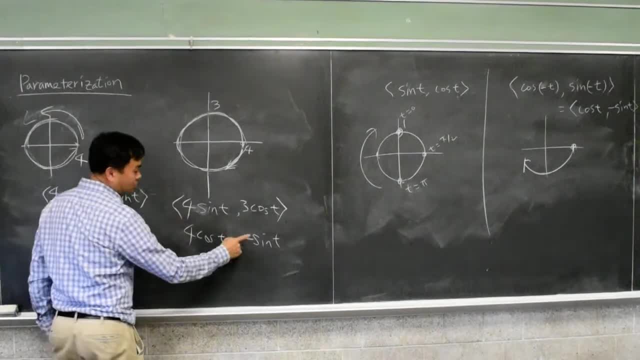 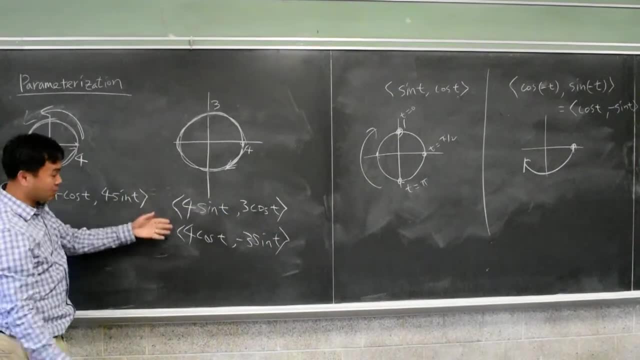 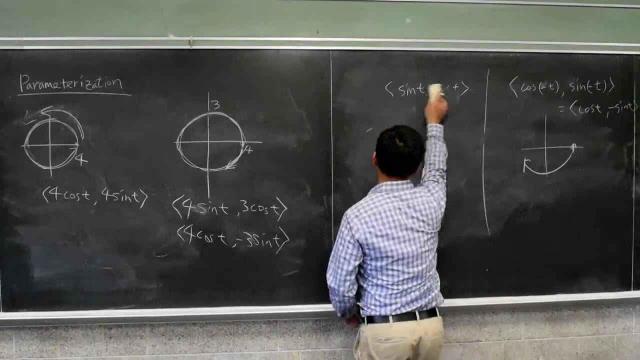 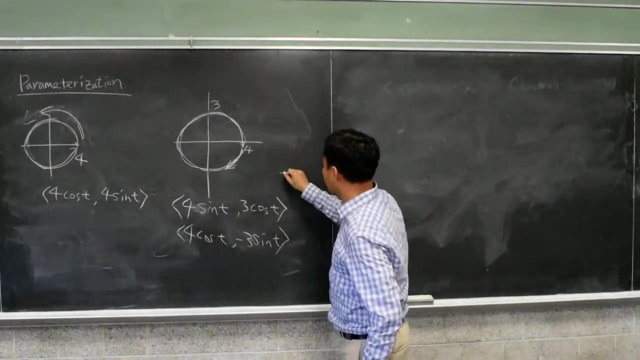 And I would multiply 4 to the x-coordinate and 3 to the y-coordinate, because I want to expand 4 times in the x-direction but 3 times in the y-direction. So either one of these will be the correct answer. Now, in all these, I omitted the fact that I want t to be 0 to 2 pi. 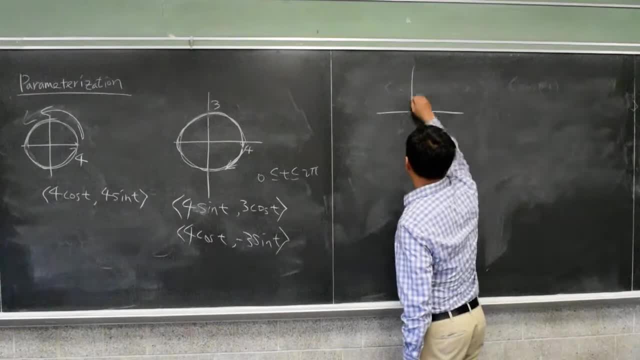 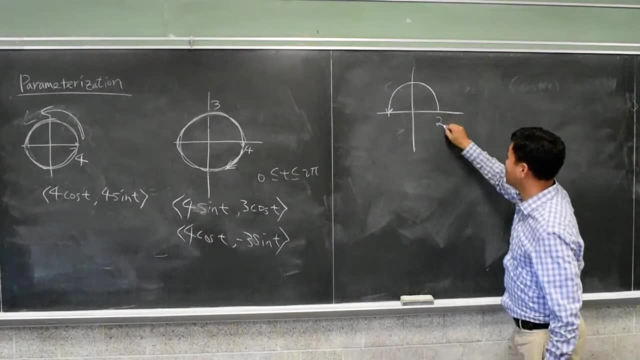 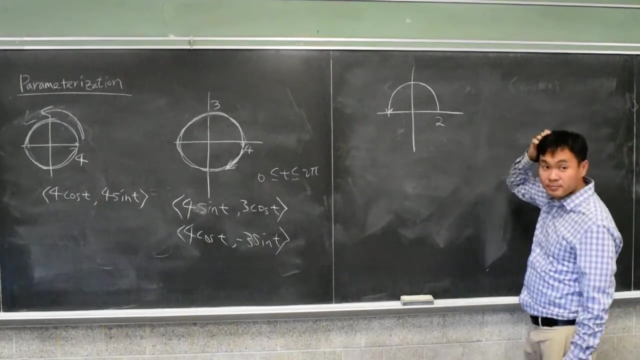 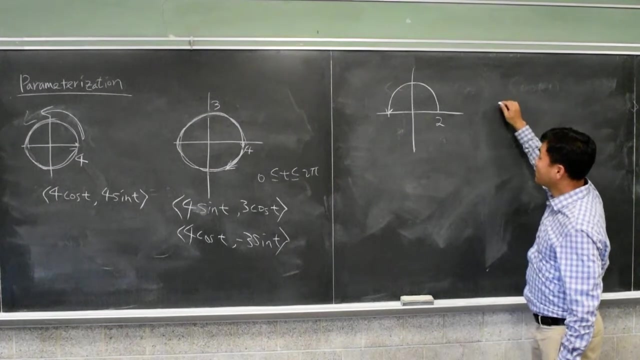 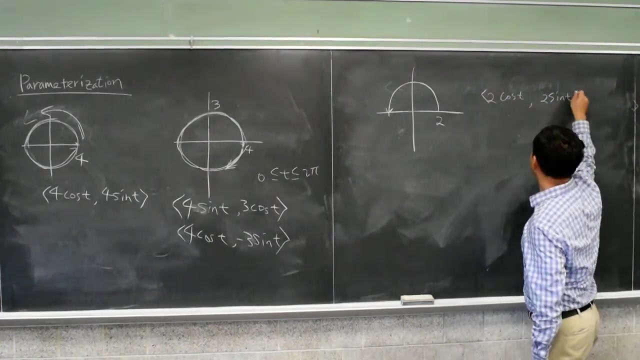 Now let's think about top half circle And let's say this is 2. It's a top half circle to how would we parameterize that one? 1. Hm, Just half it. You take cosine t, sine t, multiply by 2, like before. 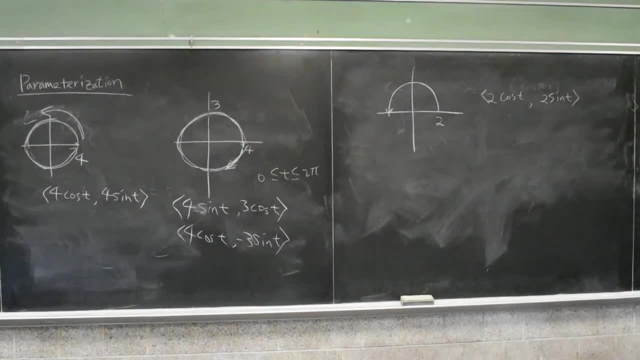 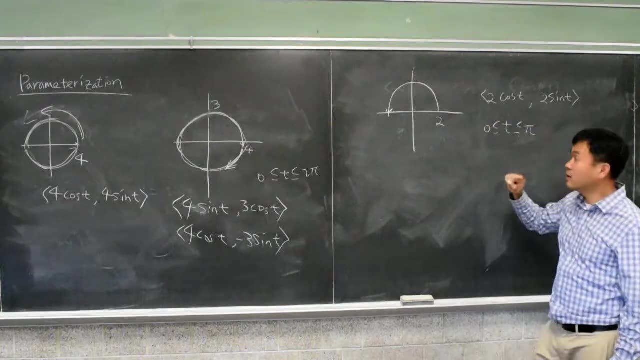 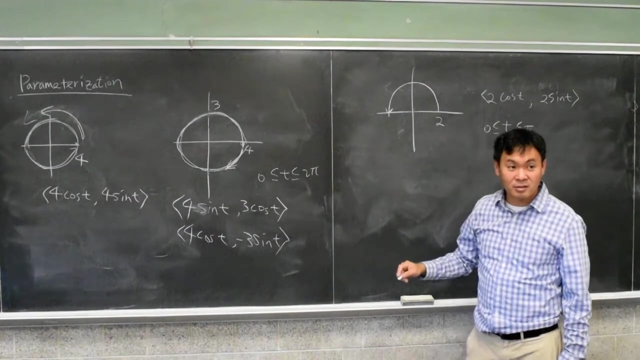 But what's changing is your t value. If your t value goes from 0 to pi, then you would only get the top half circle, So you just disregard all the values where it doesn't fall within that range. Yeah, So let's try another one. 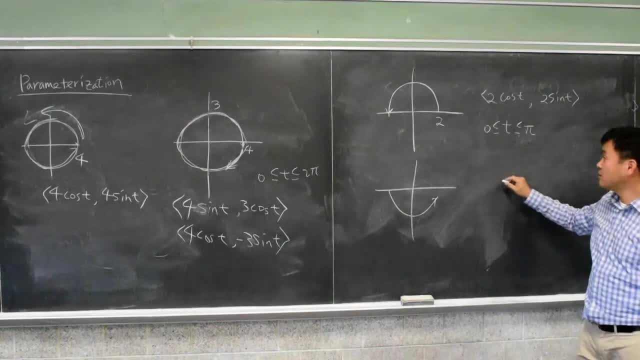 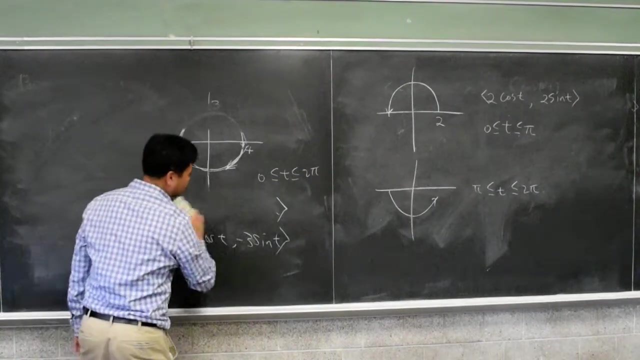 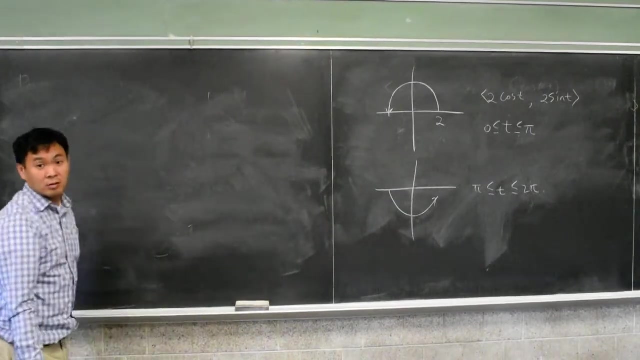 How about this one? Pi to 2 pi. Same thing, but this time it will be pi to 2 pi. Oh, Professor, Yes For this one. since it's only half, could you technically use that original parametrization with the y and x? 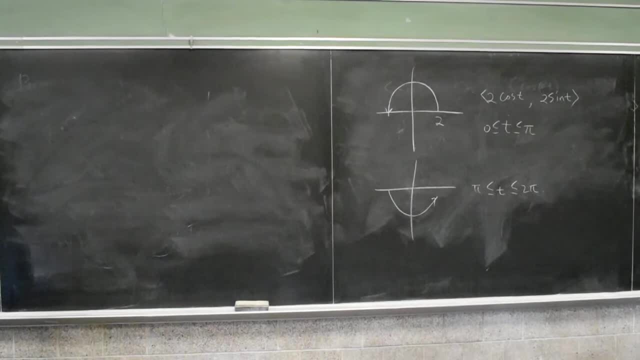 and then just take whatever top half or bottom half. Say that again, For since we're only like, if probably you can, but like since we're only getting half the circle in this one, couldn't you use the original parametrization with the x and y?